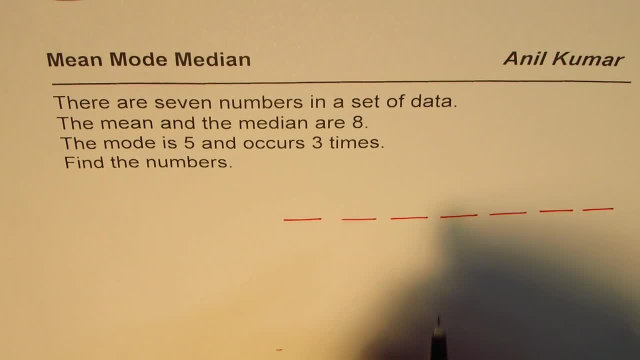 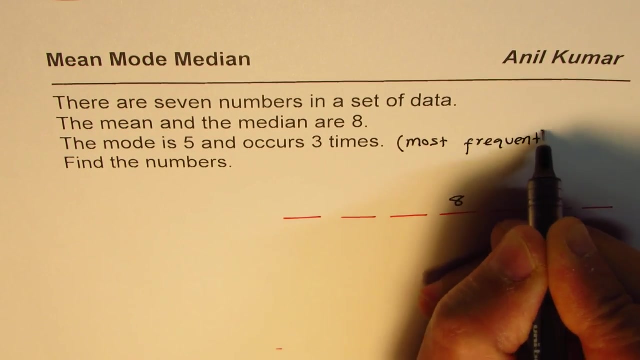 So the central value is eight. So fourth position should be eight. So we are given this is eight And we are also given mode is five, right? So mode is most frequent. So most frequent Is five and it occurs three times. So let us say we have arranged the numbers in increasing. 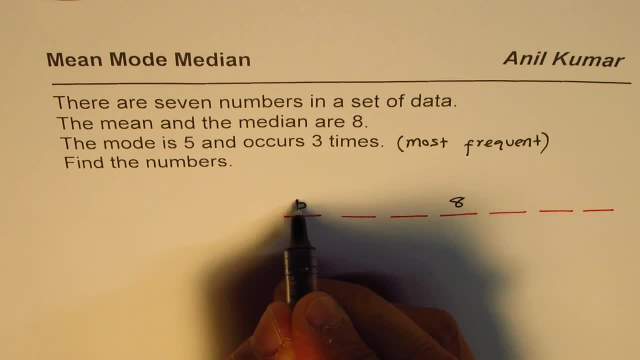 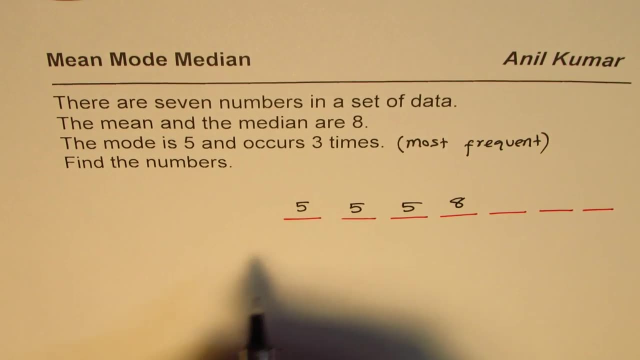 order, Then these five should occupy the first three places, Is that okay? So that is what we have. We need to find the numbers, right? So we need to find these three numbers. That is the question for us Now. I hope the question is very clear to you. You can still pause. 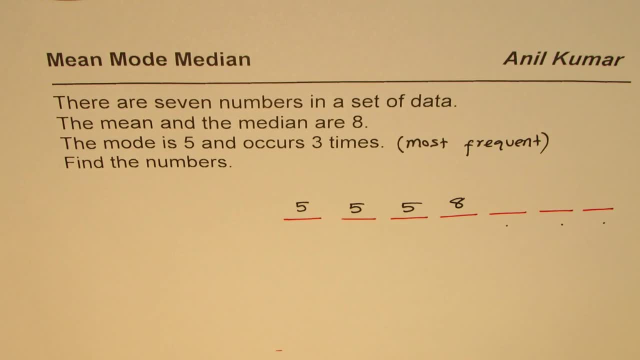 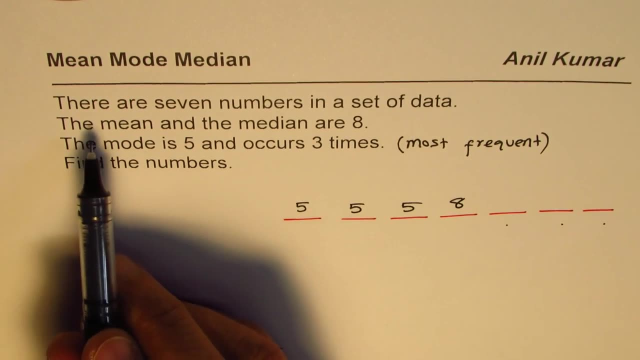 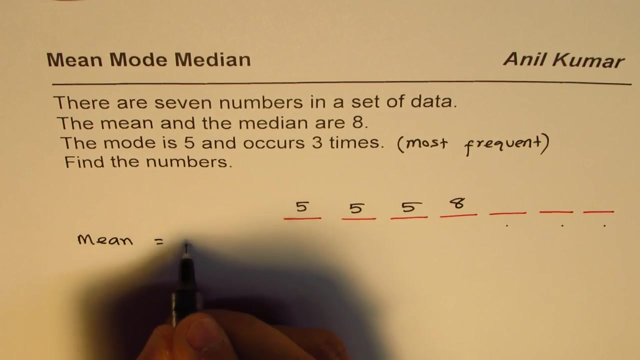 the video and answer the question. How do we get these numbers? Let us read the question. There are seven numbers in a set of data. Okay, The mean and median are eight, So we are also given mean. So we are given mean is equals to eight And the number of numbers is seven, right, So what should be? 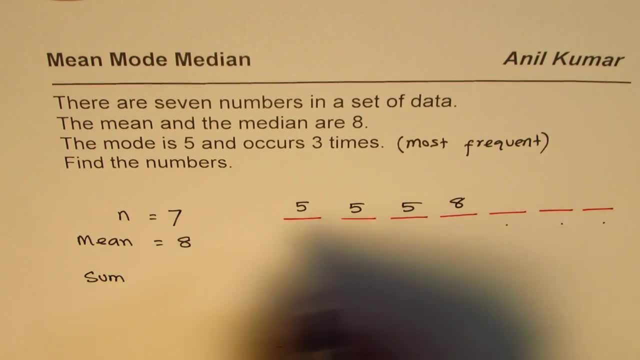 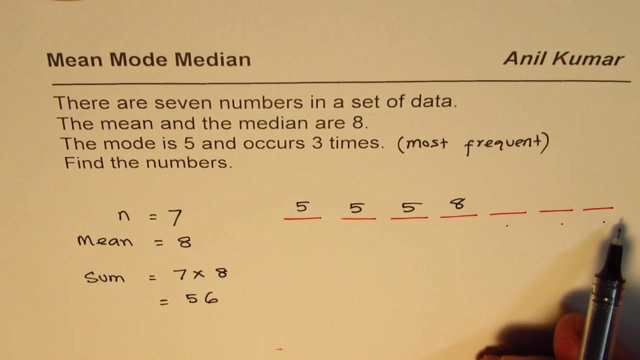 the sum. What should be? sum total of all the seven numbers? It should be mean times the number of numbers, right? It should be seven times eight. So the sum should be 56.. Does that give you a clue? So when you add these numbers, we should get 56. And also, these numbers should be greater. 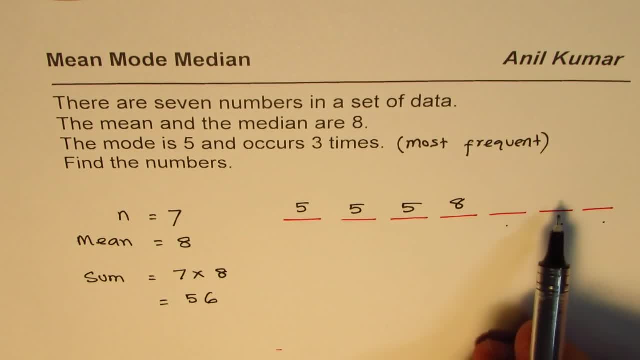 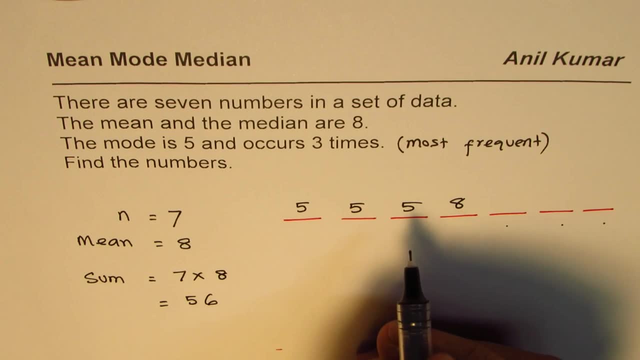 than eight. We are not expecting any number to be like three of one kind, since the mode is only five. Now I think it should be simpler. So let us find what is the sum of these three numbers, right? So sum of these three numbers should be 56.. 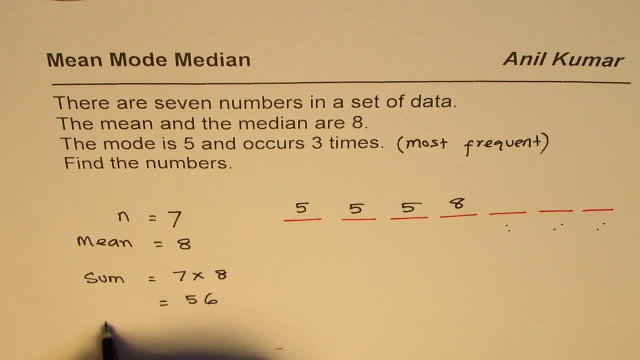 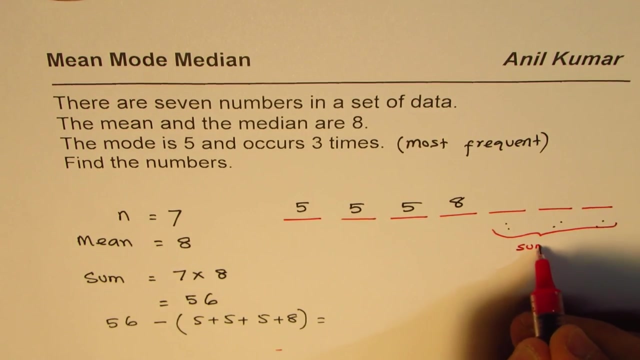 What is the sum of these three numbers? Okay, So let us say these three numbers should be 56. take away 5 plus 5 plus 5 plus 8, right, That is sum of these three. So what we are trying to find is sum of these numbers, right? 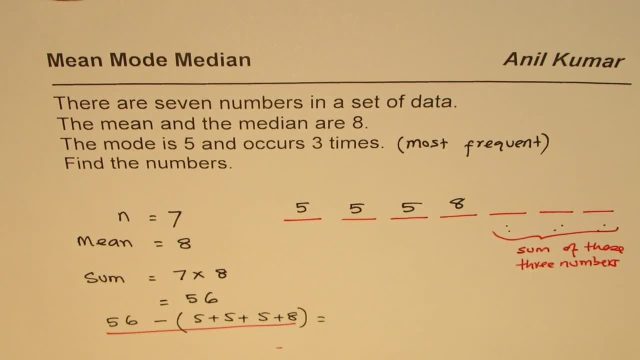 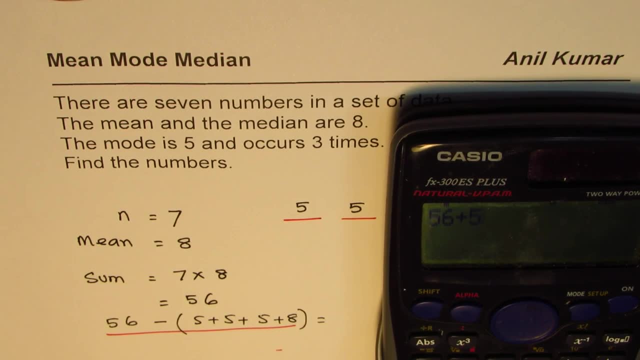 Okay, This is what we are trying to find here. Okay, So, which is? let us use calculator. So we have 56, take away 5, take away, I mean 56, take away 5, take away 5, take away 5 and take away 8.. That gives us 33.. Okay, So, that gives us. 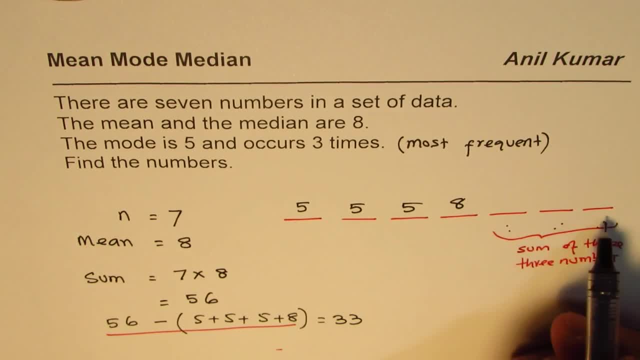 33.. So these numbers should be such that their sum is 33.. Do you get an idea? So some of these numbers should be 33.. So that gives us all possible combinations. Do you get an idea? Some should be 33.. Okay, At increasing order. Okay, So one way is 33, we could take. 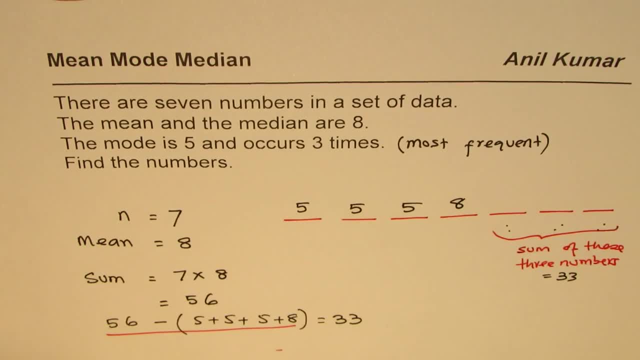 11 here. So one combination could be: let us write down possible combination. One combination could be: I could take 11 here 33, let us divide this by 3.. We get 11, right: 11,, 11,, 11.. That. 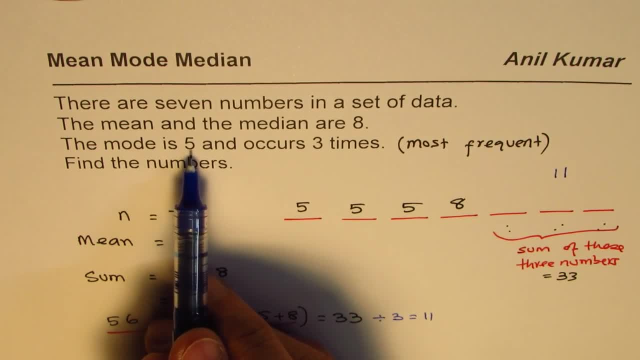 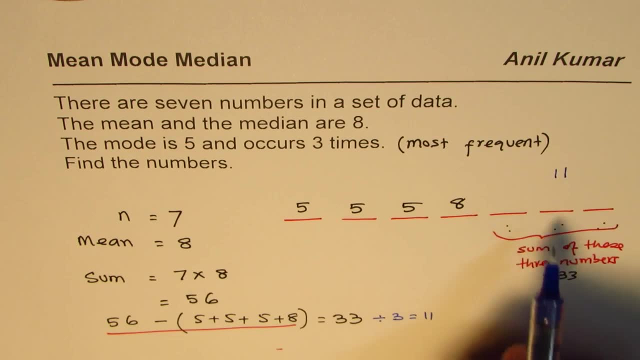 could work, But no mode is 5.. If I take 3, 11s, mode will be also 11.. So 11 cannot be the number. But well, 11 is my mean of these 3.. So the numbers could be 10,, 11,, 12.. Does it make sense, Correct, So? 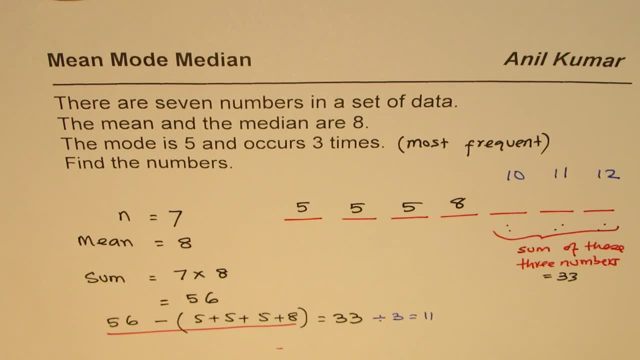 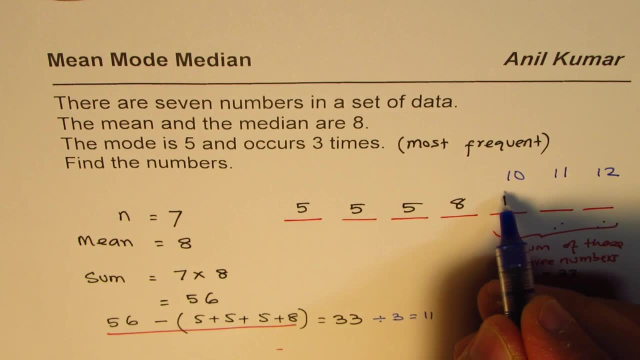 it could be 10,, 11,, 12. So that could be one of the combinations, right? Or I could take 10 two times, right? So I could take 10.- 10. And then it becomes 20. And we need 33.. So the other number could be 13.. So that is how we. 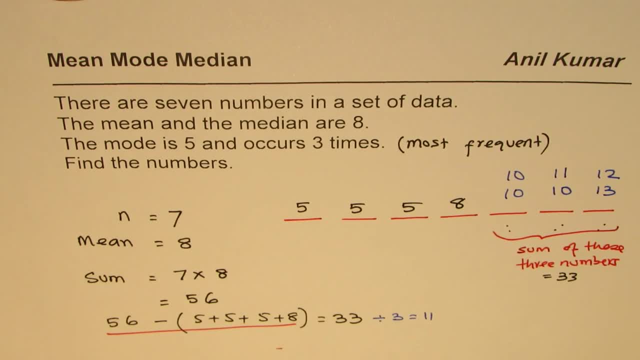 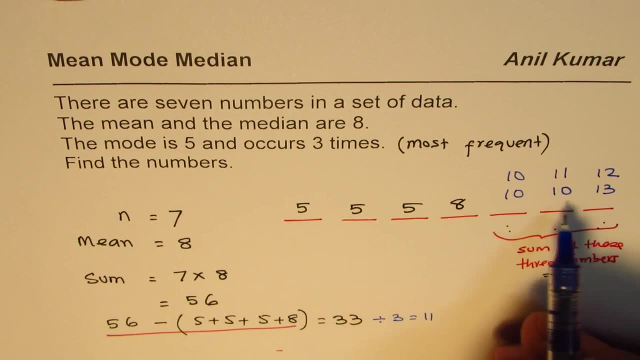 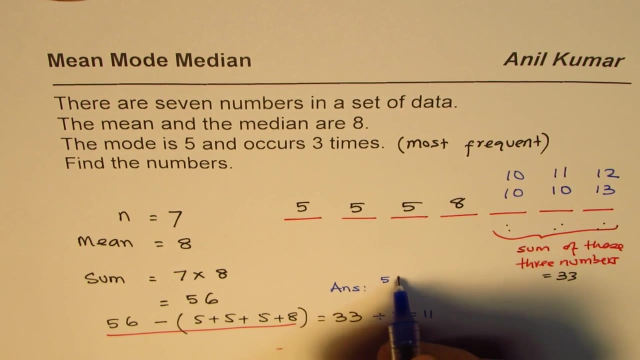 can get different combinations. Do you get it So? likewise, you can find all possible combinations also, right? So our answer could be either one of these, So the 7 numbers could be. So the answer which I am writing here is the 7 numbers are 3, 5s, 8.. And then the other number could be: 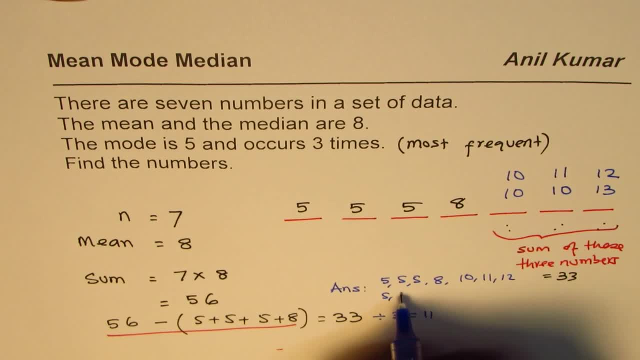 10,, 10,, 11,, 12.. Another answer could be 3, 5s, 8. And it could be 10,, 10, and 13.. Correct, So likewise we can get different combinations. We could use other combinations also, So.